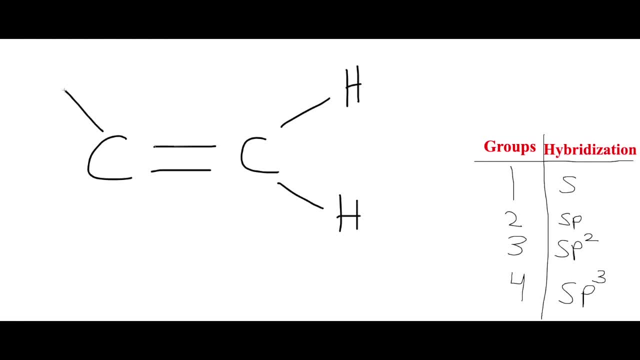 We've got two hydrogens And you are asked to know what is the hybridization for this first carbon and also the second carbon, right? So this is where the groups in hybridization come into place, right? So if you have one group meaning one bond, it's an S. If you have two groups, it means you have SP. 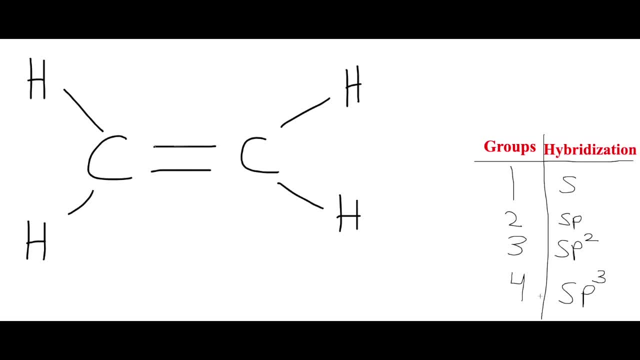 If you have three groups, it's SP. If you have four groups, it's SP2.. If you have four groups, it's SP3.. So what does this mean? It means that if you look at the first carbon right, first carbon, it's connected to how many bonds. 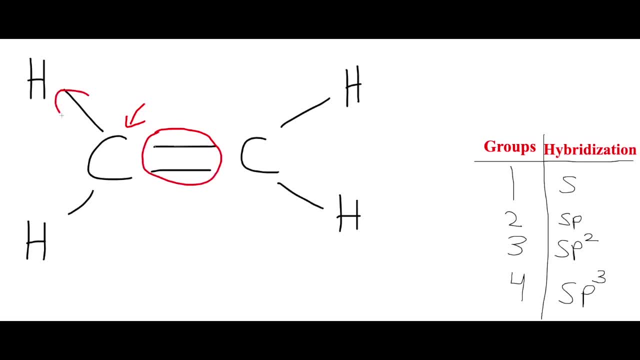 So we've got one, two and three. alright, So that's three bonds. Three bonds is right here. So it's three bonds, three groups, which would be SP2, right, So this is SP2. right here for this carbon. 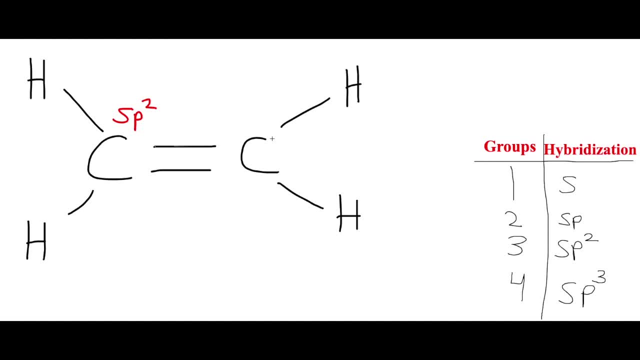 Now, if you look at the second carbon and determine its hybridization, we know it also has one, two, three, three groups. Three groups is SP2 hybridization. So we also know that this carbon is also SP2, right? 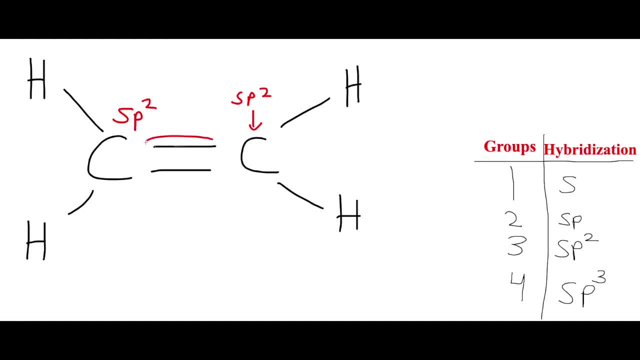 So groups, meaning that how many bonds it has, right. So we don't count individually, but we count as a whole if it's connected to it as a whole, right. So let's go to the next problem here. Say, we have this example right here, right? 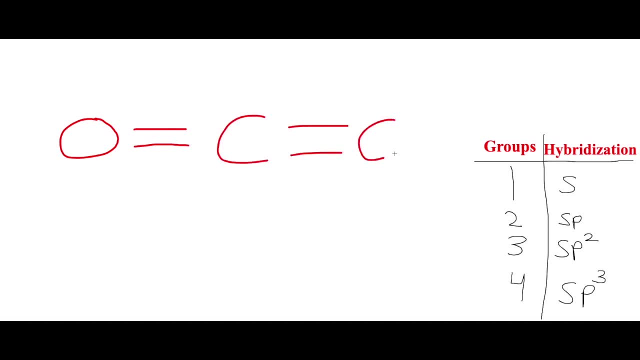 So let's say we have this example right here, right, And we were told to know what is a hybridization for this oxygen right here, this oxygen right here, What is a hybridization for it. So we count how many bonds it has, right. 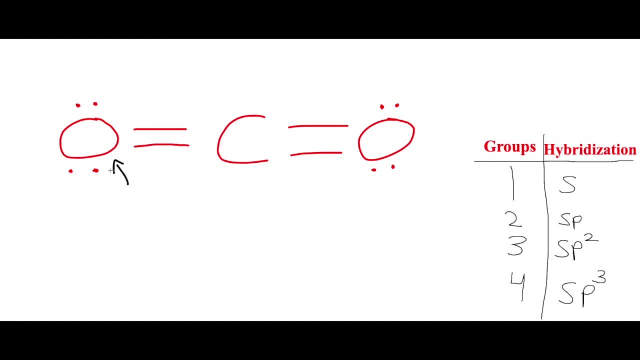 So Bone pairs count as one bond as well. So that's one group. So that's one, two, three. So again it has three bonds, so three groups, meaning it's SP2, hybridization, orbital right. So this is SP2.. 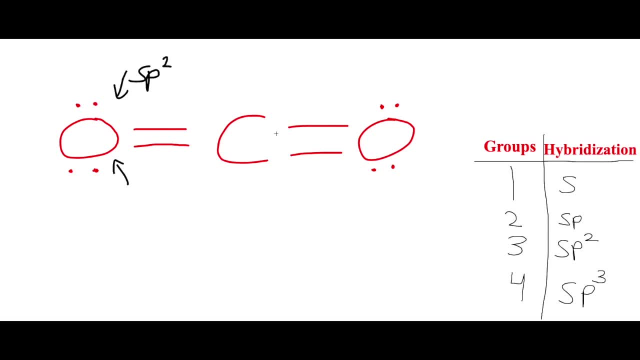 Now this carbon right here, the middle carbon, how many bonds is it connected to? So we know carbon can only have four bonds in total. So there's two right here and then two right here, but it counts as one. So one and then two. 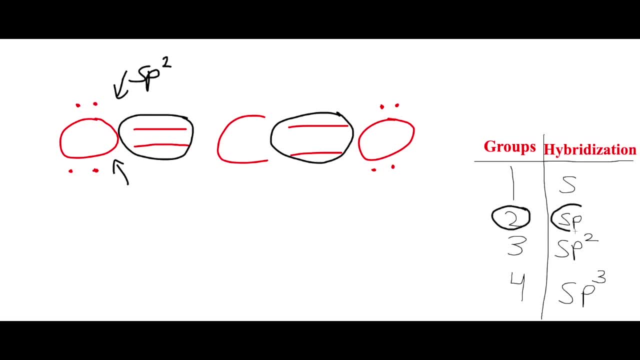 So it's two, two groups, meaning this is SP, hybridization orbital. So this carbon right here is SP, SP. Now, finally, for this last oxygen, over here, it's connected to one bond, two bonds, three bonds right. 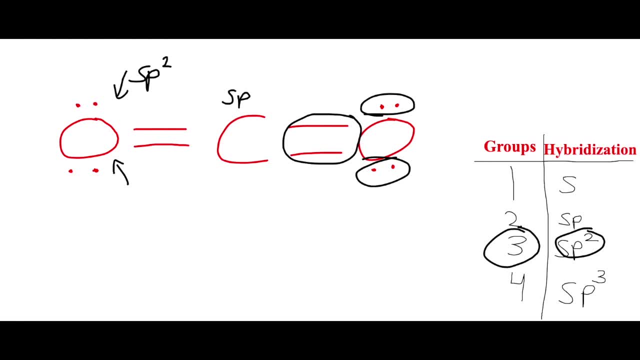 So three groups, Which is SP2.. So SP2, right here. okay, Let's do another example. Okay, Say, I have this structure right here, Right, And we were able to determine the hybridization for it. So let's go with the carbon first. 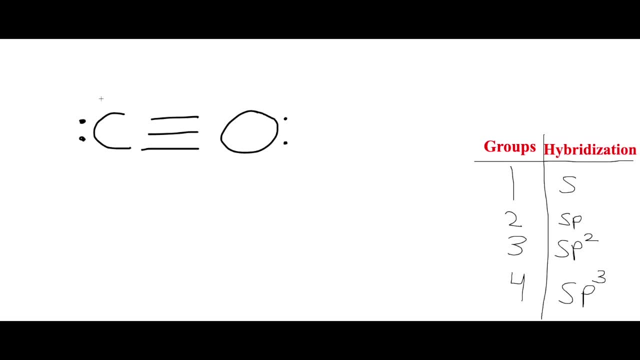 Right. So this carbon right here has how many groups to it? So one group, It has two groups right here, So two groups, meaning it is SP, precisely. So this carbon right here is SP. Now, for this oxygen, we have one and we have two. That is also SP for it, And so we'll do it. It will be SP over here. I believe Yes. 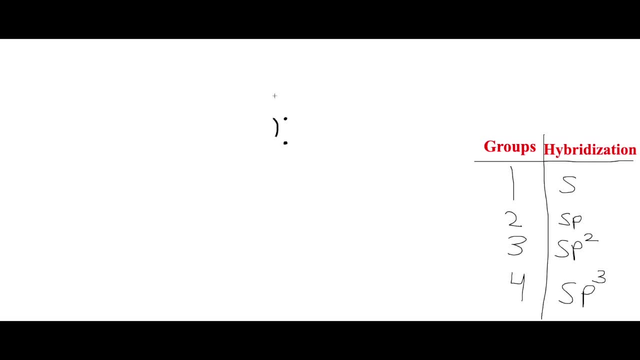 All right, Let's go back. Let's do another example. Now say, we have this example right here: Oxygen with two lone pairs, a double bond to carbon and connected to a hydrogen- Two hydrogens, All right, All right. So let's start off with carbon right down the middle. This carbon is connected to what It's connected to one. 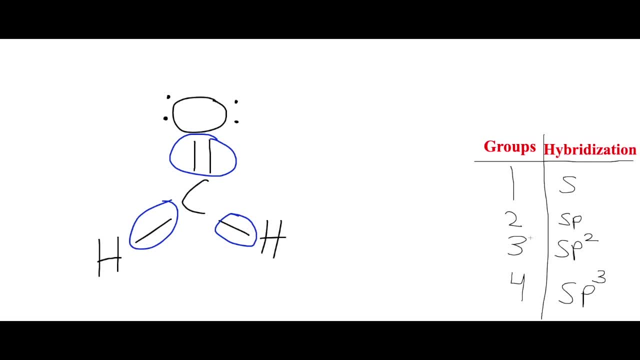 Two and three, Three groups, Right, Three groups. So that's SP2.. Okay, So this carbon right here is SP2.. Now, what about this oxygen over here? Well, it's one, two and three. It's connected to three groups. It's also SP2.. 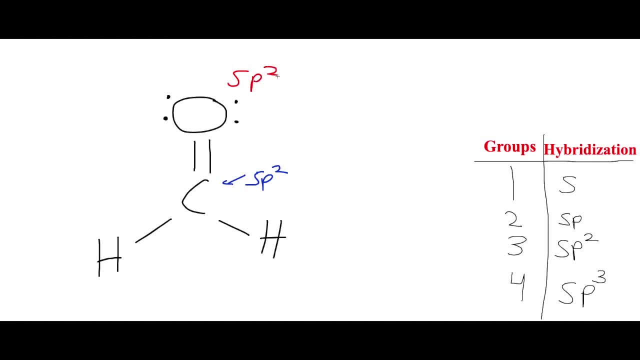 SP2.. Okay, Let's do another example. Say we have this, We have water, Right Structure for water, Water, All right. So we want to determine what's the hydrogenization for this oxygen, And so what we do, we count how many groups it's connected to. So we've got one group over here, Two, three and four. 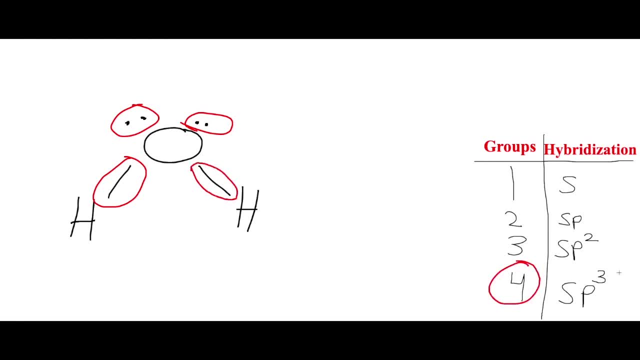 We've got four groups connected to it, So it's four groups, which is SP3.. Okay, So this oxygen is SP3.. Now let's see these hydrogens. I mean, for the most part, your professor doesn't have to tell you. 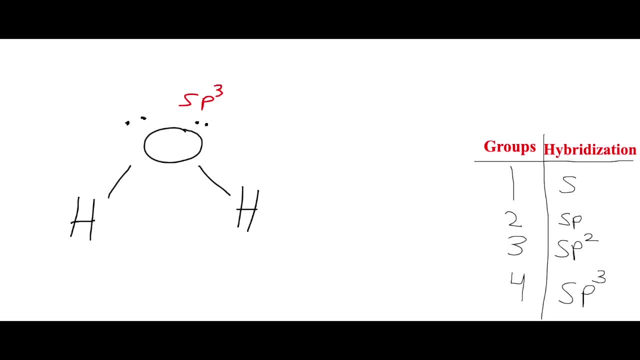 He doesn't want you to know. the hydrogen is very simple, But if we had to do it, we see that it's connected to only one group. Right Both hydrogen is. So if this hydrogen is connected to one group, the one group right here would just be S.